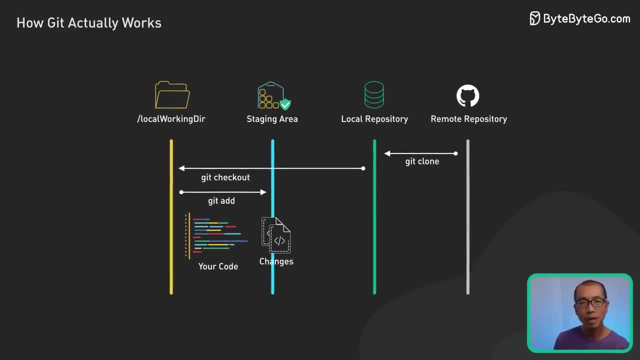 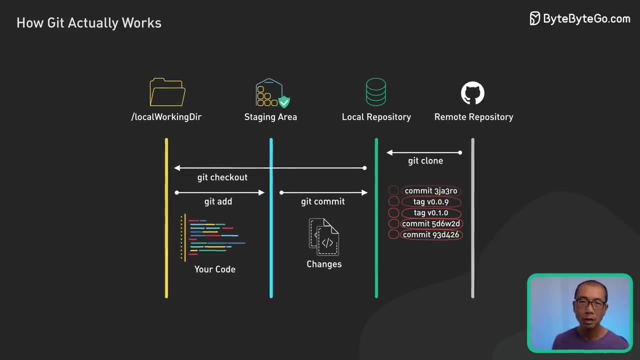 a checkpoint where your code changes are gathered up and ready to be finalized. The next step is to use Git commit, which takes a snapshot of the staging area and saves it to your local repository. This locks in those stage changes by creating a permanent record that you can refer back to like a snapshot in time. 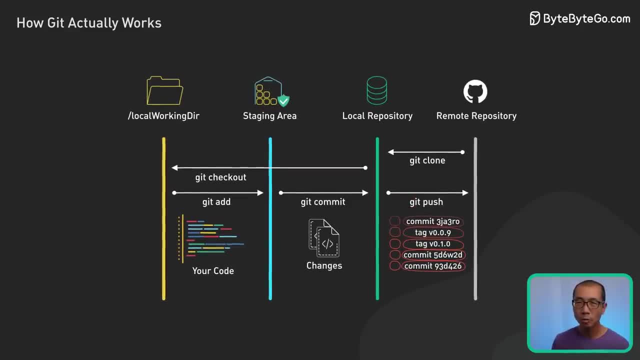 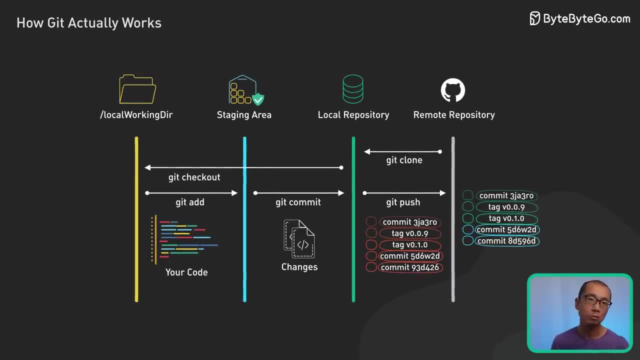 Your code doesn't just stay on your local machine. When you are ready to share your progress with the team or back up your work, you use Git push to send your commits to the remote repository. This is often a shared server where your team can collaborate. 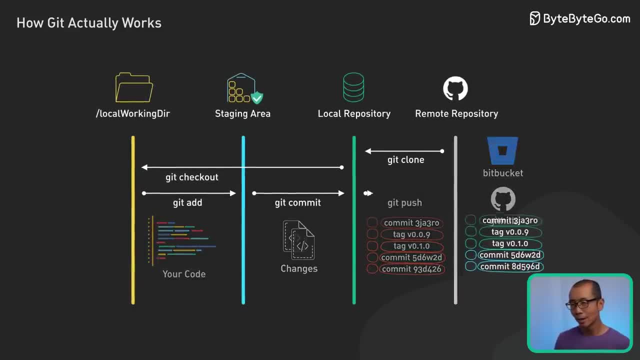 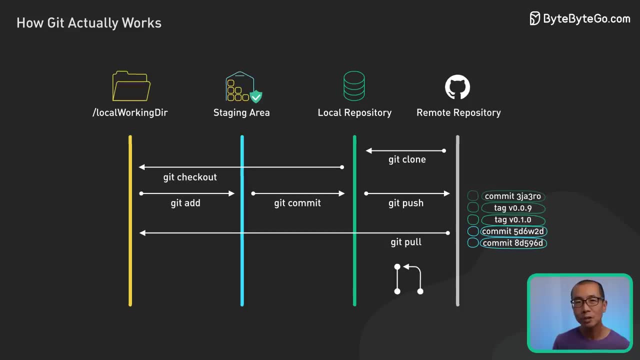 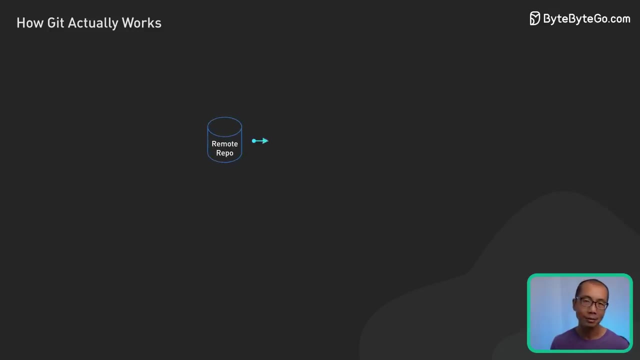 like GitHub or Bitbucket, Collaboration in Git is a two-way exchange. To integrate your teammates' work, you use git pull, which fetches changes from the remote repository and merges them into your local repository. It combines two commands: git fetch, which grabs the latest updates. 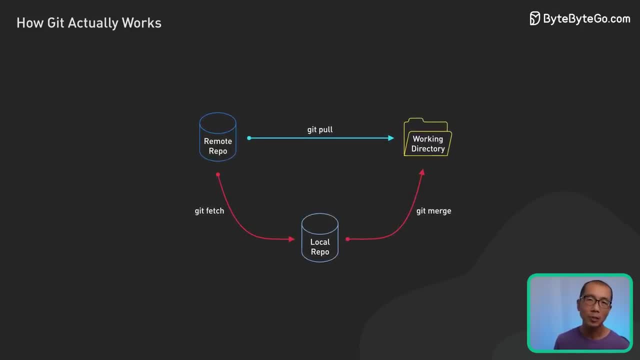 and git merge, which integrates these updates with your work. There are times when you need to switch contacts, perhaps to fix a bug on another branch. That's where git checkout or git switch comes in. It allows you to switch between different branches to work on specific features. 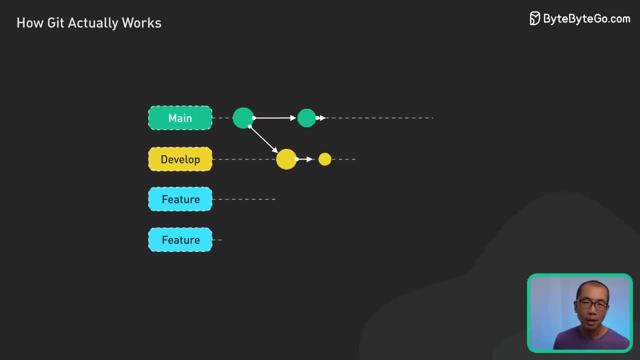 Git branching allows you to diverge from the main code base to develop a new feature without impacting the main code. Some key concepts include: creating a new branch with git branch, switching between branches using git switch, merging branches. together with git, You can also work with git merge or resolving merge conflicts. 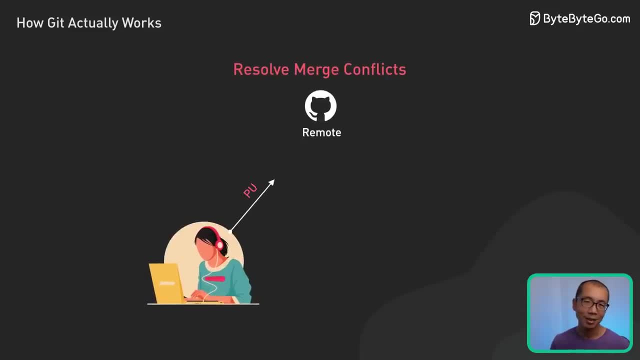 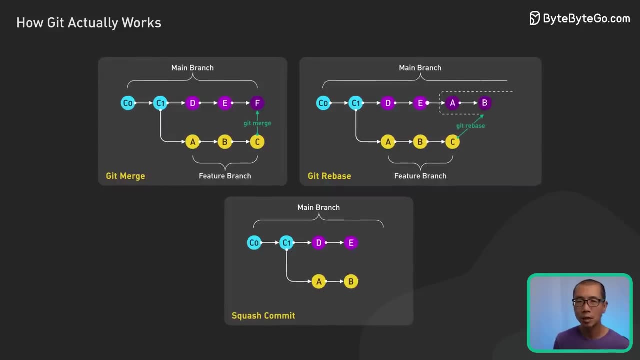 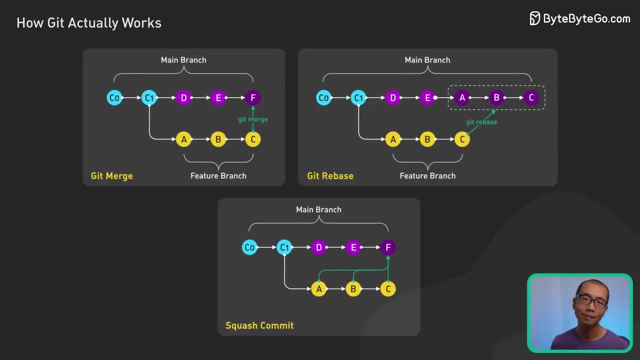 when changes overlap, Branching enables isolated development and collaboration workflows. There are more nuances when merging or rebasing changes from others or managing branches. We have a dedicated video on merging and rebasing that we encourage you to watch. Many developers use graphical git tools like GitHub Desktop and SourceTree. 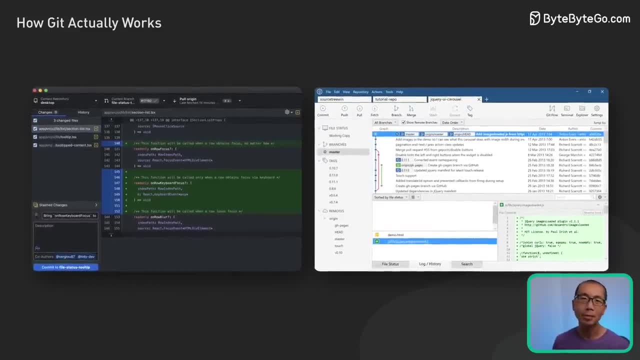 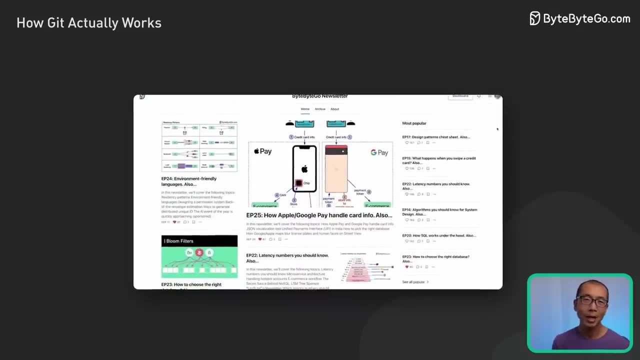 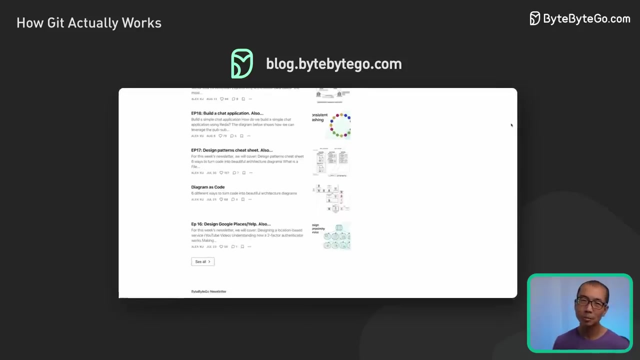 These tools provide visual interfaces and shortcuts to common commands. They can help new users get started with git more easily. If you like our videos, you might like our system design newsletter as well. It covers topics and trends in large-scale system design, trusted by 500,000 readers. 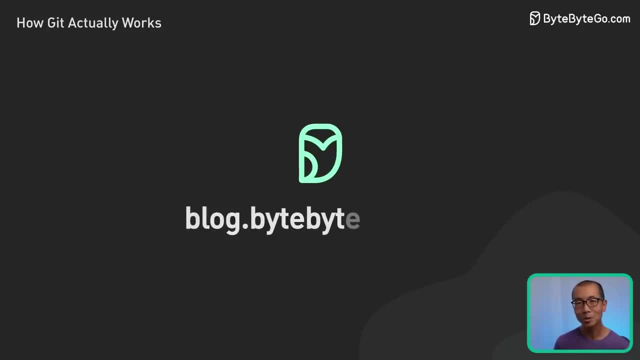 Subscribe at blogbybygocom.